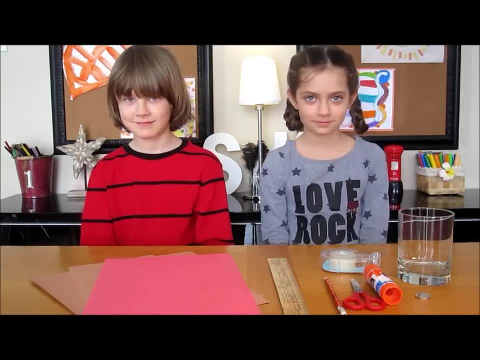 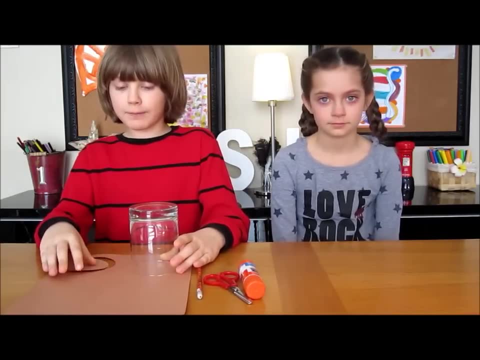 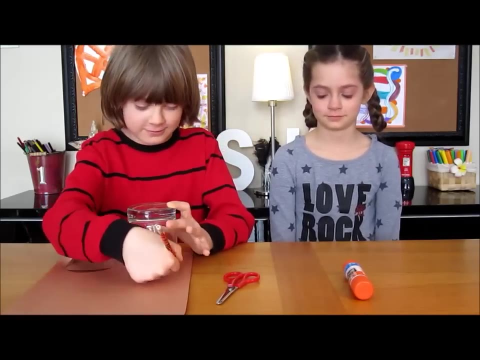 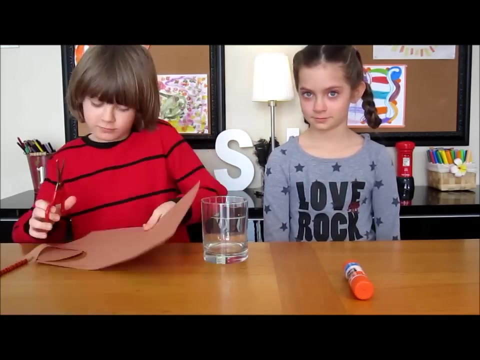 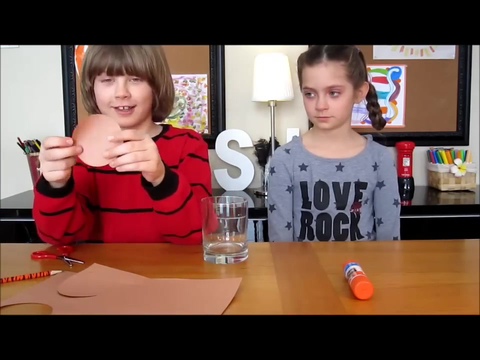 scotch tape, a penny and a glass. First, put your glass on the construction paper and trace it. Once you've traced it, cut it out. When you're done cutting it out, it will look like this And it will fit perfectly in your glass. 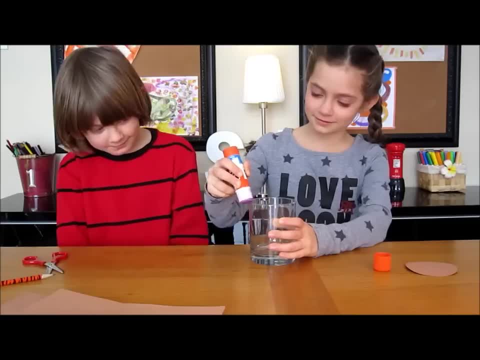 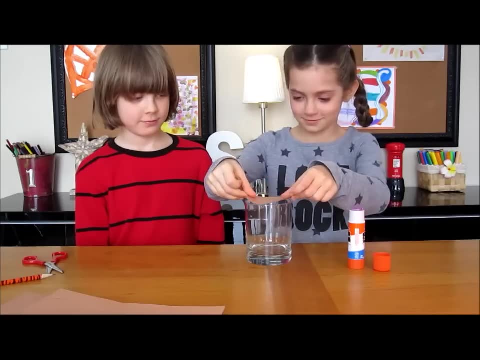 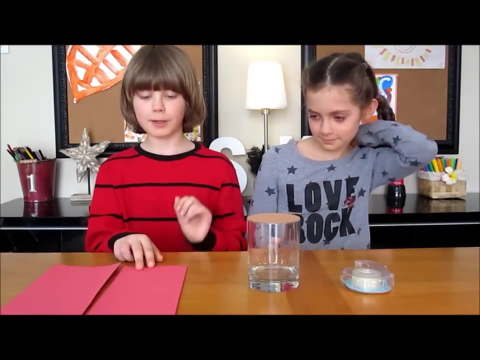 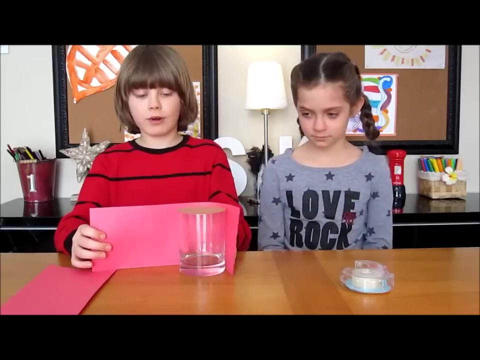 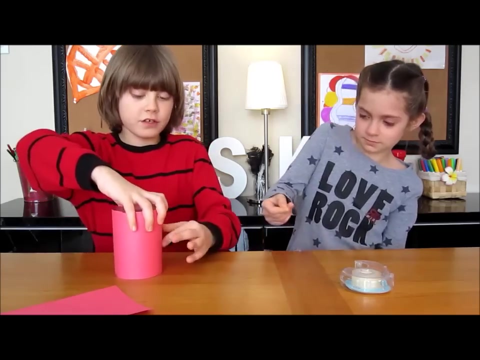 Second step: you put some glue around the glass And then you put your circle on it. Take your one color paper and cut rectangles the same size as your glass. Then take the rectangle and wrap it around your glass And fix it with scotch tape. 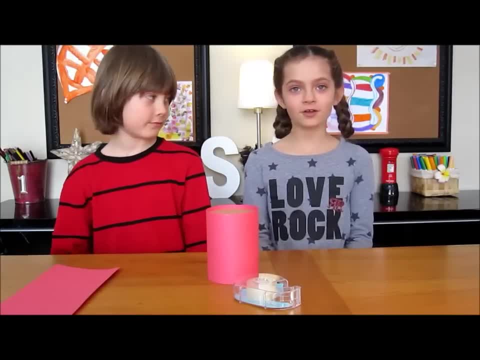 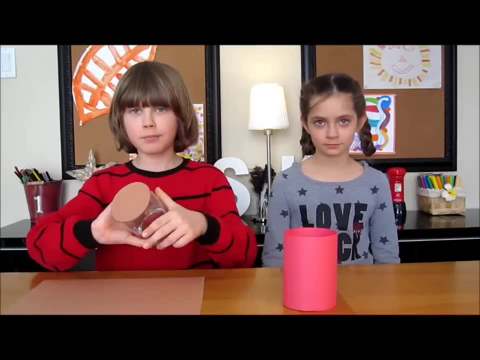 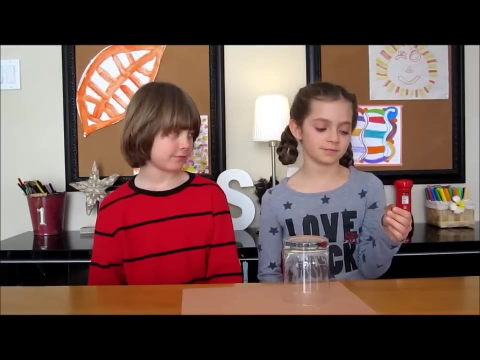 And that's it. Now you're ready to impress your friends and family with your magic trick. Let me show you how it works. Before anybody sees, put your glass on your construction paper that serves as your mat. Now tell your audience that you're going to make your coin disappear. 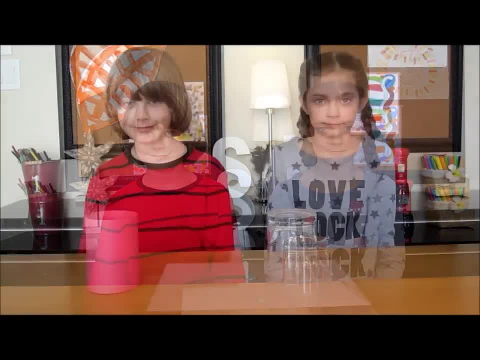 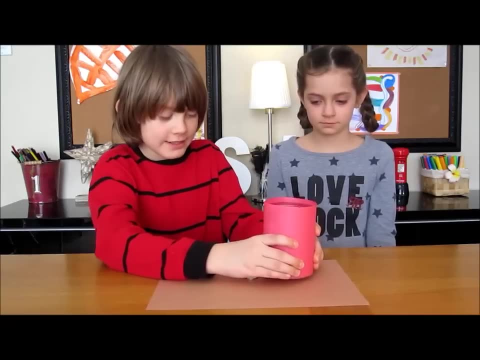 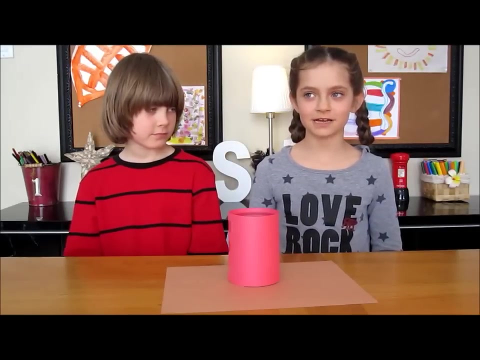 Put the coin on the mat beside your glass, Take your tube and put it over your glass in front of the audience, Carefully. lift your glass and your tube and put it over your coin. Once you did that, pronounce a magic spell like this: 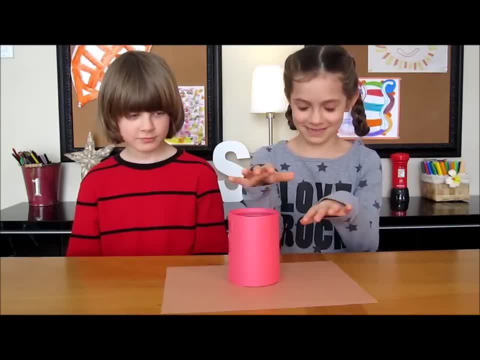 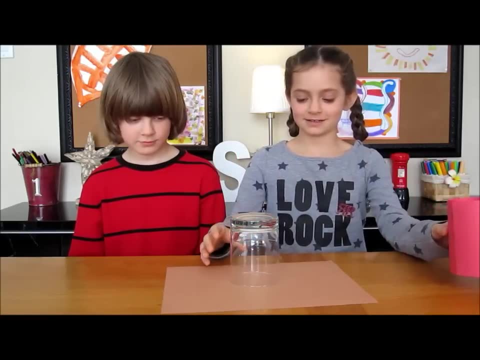 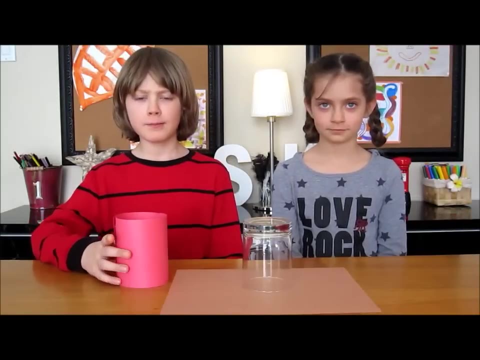 Abracadabra, abracadabra, make your coin disappear. So then lift your tube up and then say, ta-da, Your coin disappeared. Tell your audience that you're going to be making your coin reappear. Put your tube over your glass. 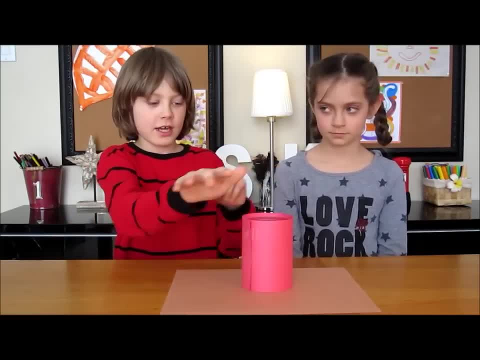 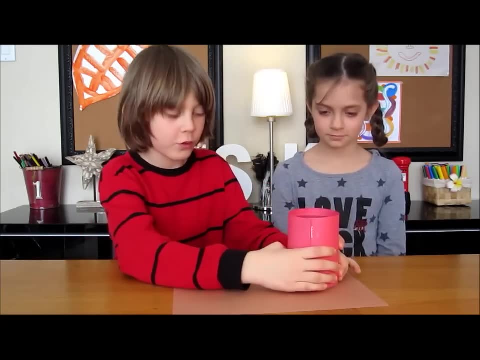 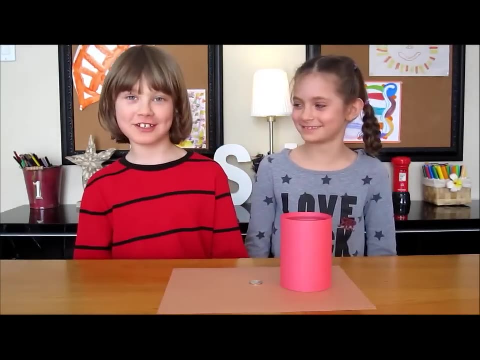 And say the same spell that you said: Abracadabra coin, come back, And your coin. and your coin will come back, Ta-da. Now it's your turn to try this magic trick and have fun. See you next time. Bye.